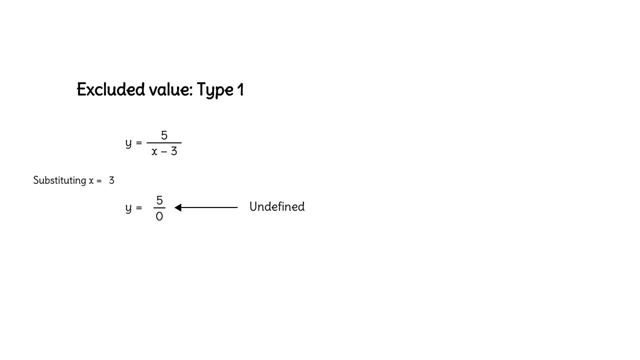 5 over 0?? That's undefined. We can't substitute 3 for x in this function and get a defined result, so 3 is the excluded value. The reason is that an x of 3 results in division by 0.. 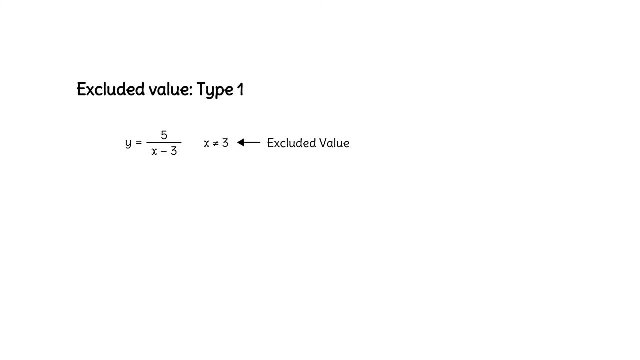 How does that impact the graph of this function? If we substitute x-values that are close to 3, like 3.1,, we get a large positive y-value of 50.. The same is true when we substitute 2.9.. We get 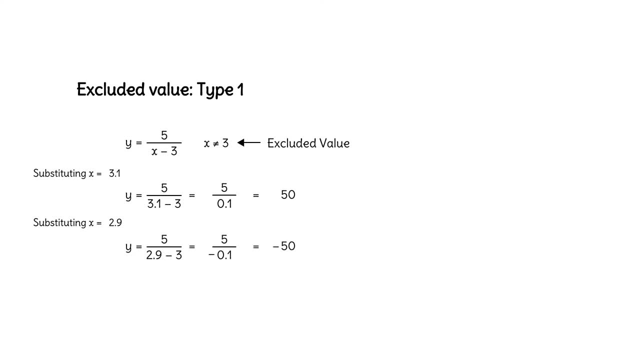 a large negative y-value of negative 50.. The closer we get to 3,, the larger the y-values this function returns. We can see this in the graph of: y equals 5 over x minus 3.. There is no y-value for an x-value of 3, but the graph balloons to infinity for x-values close. 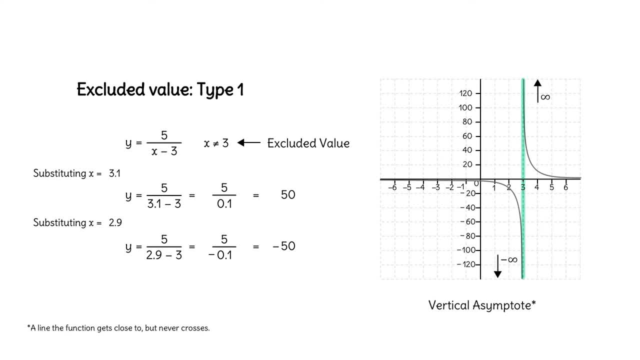 to 3.. You might recognize this feature as a vertical asymptote. You'll see these frequently when graphing rational functions. Remember, if a value results in division by 0, it's an excluded value and it results in a vertical asymptote. 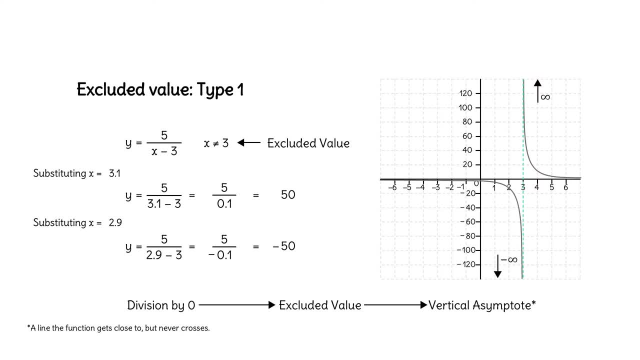 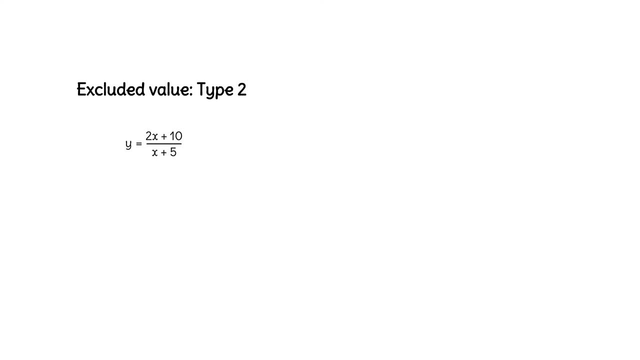 for the graph. This is the first type of excluded value we sometimes see. So what's the other type? This rational function will demonstrate it. Can you think of a value for x that might be excluded? What value of x would make? x plus 5 equals 0? Negative 5.. 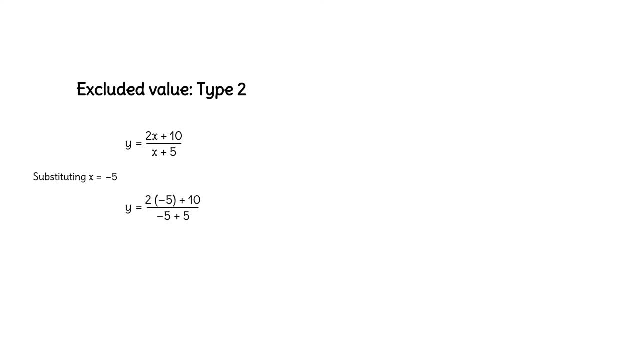 But something very strange happens: when we substitute negative 5 for x, We get 0 in the numerator and in the denominator. What is 0 over 0?? It's also undefined. So negative 5 is an example of the second type of excluded value. 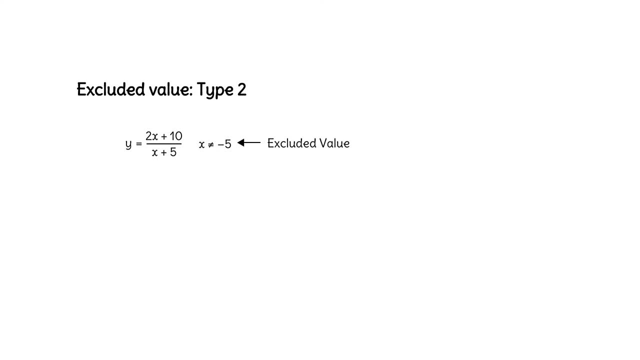 How does this type of excluded value impact the function? If we factor the numerator and denominator of this rational function, we can cancel x plus 5.. So this function simplifies to: y equals 2, but we can't forget our excluded value of negative 5.. 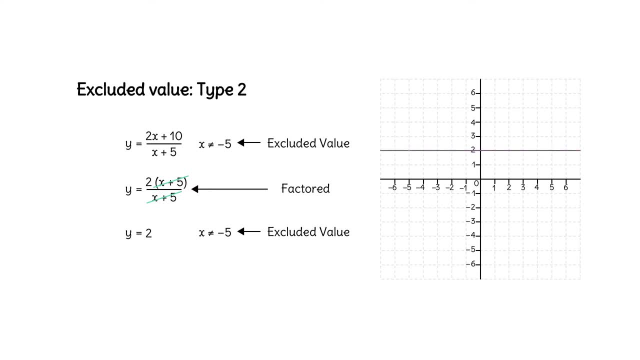 The graph of y equals 2 is a horizontal line, but at the x value of negative 5, we graph a hole, an open circle, because negative 5 is an excluded value. Remember, if an x value results in 0 over 0, it's an excluded value.